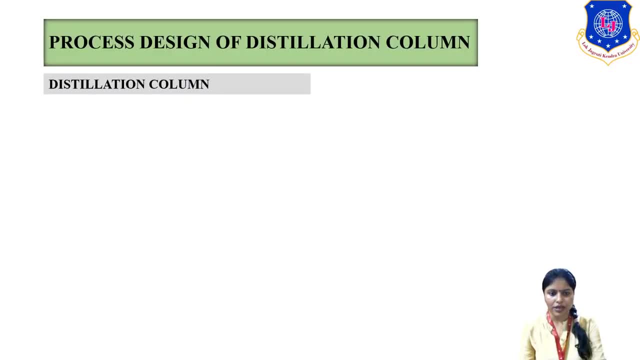 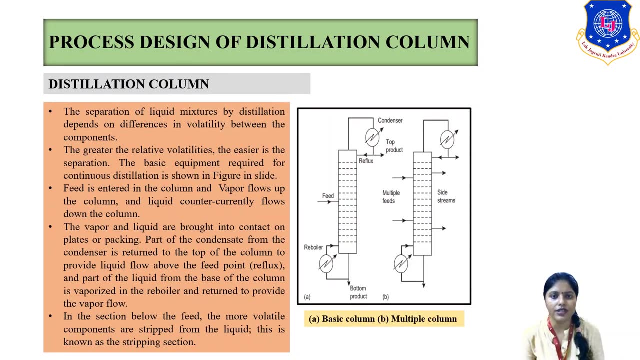 Column Design. So the chapter name is Process Design of Distillation Column and today we are going to discuss about the how to design the distillation column. So I know, before starting the designing of distillation column, let us revise the how. what is distillation? 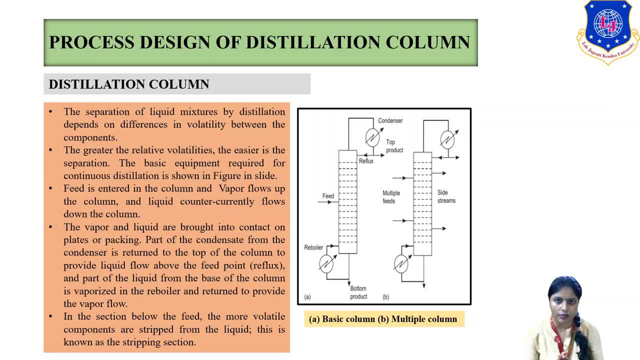 column. I know you have learnt the distillation column in semester 5th- mass transfer, operation 1, but let us have a quick revision of distillation column. So, starting from the what is distillation column? Distillation column is a separation. 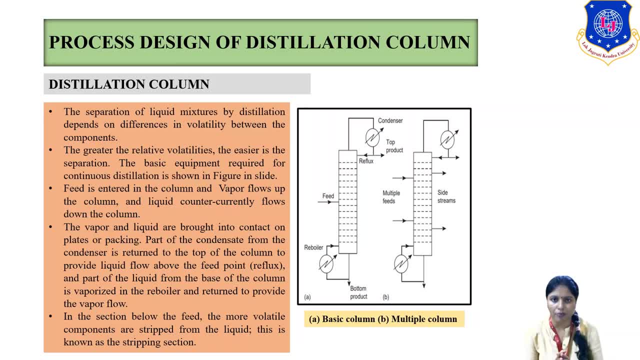 equipment where the two liquids are been separated from each other on basis on their boiling point. Note the word boiling point because it is an important word used for the definition of distillation column. So if the two liquids have the different boiling points, they have been easily separated. 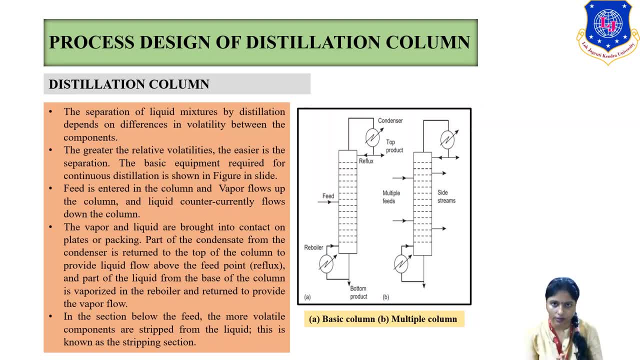 from the distillation column. There are two types of distillation column, like tray tower or the packed column, Right. so what will happen with the tray tower column is that the trays will be kept in between the column. And what will happen with the packed tower? 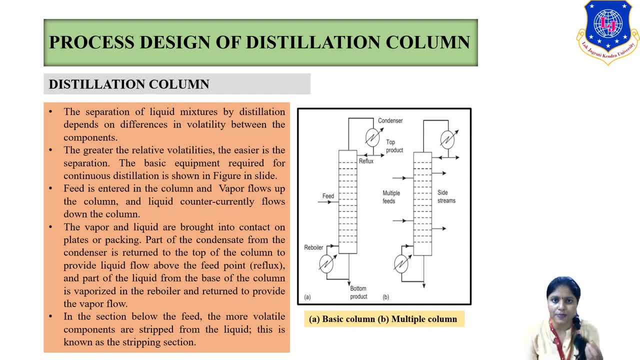 Packed means some packing type of material has been kept in between the column, If you column Packed tower also has been differentiated into two parts. First is random packing and second is regular packing. So what is random packing? Random packing is a packing of irregular shape. 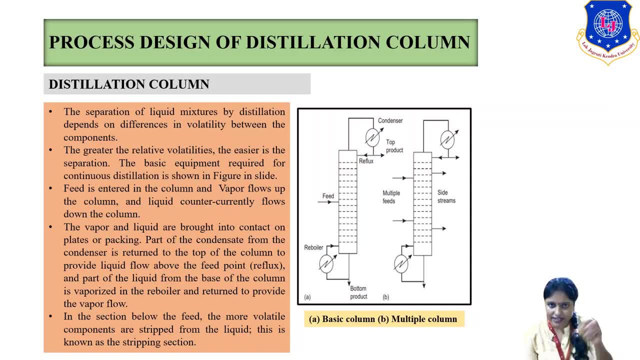 The packing will be of irregularity, so that been placed in the in between the column and that is known as random packing. And what is a regular packing? Regular packing is the packing is of regular shape, So the shape which is used for the bits or the packing material is of regular. 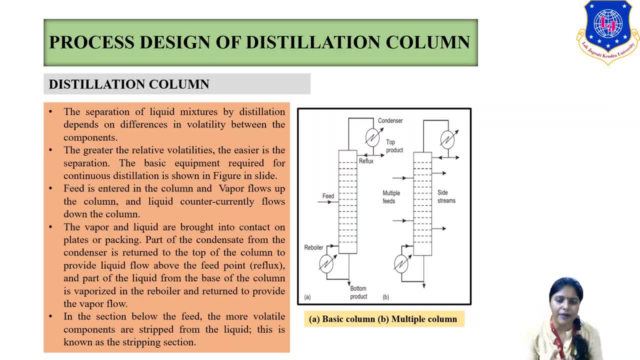 okay, So what will happen in the random and regular packing? that in the random packing the there will be high valu pressure, high drop of vapor pressure and it is of low cost, but the channeling problem will be there in the random packing, While in the regular packing there will 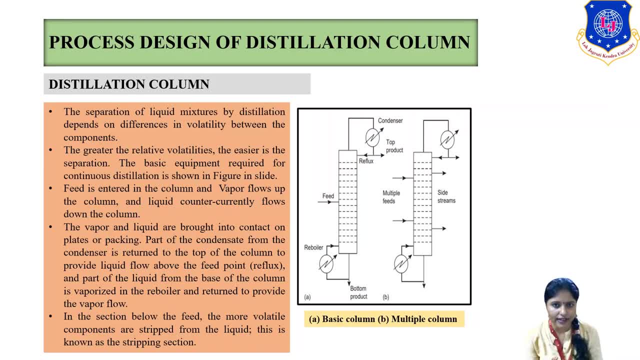 be no problem in channeling. So what happens in the channeling? that the, when the liquid comes and the liquid will liquid and the gas, the two liquid, will go not on the between of the packing, it will go on the side of the column right. so that is a problem of channeling. so in 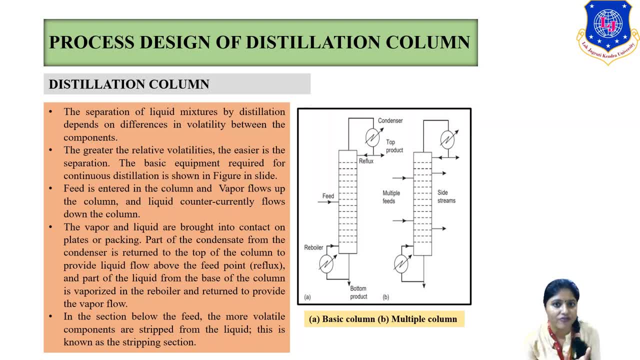 the regular packing, you won't be seeing this type of channeling, while the random packing the channeling problem is always there: that the regular packing is of high cost while the random packing is of low cost. so in this figure I have shown that there are two types of column right. 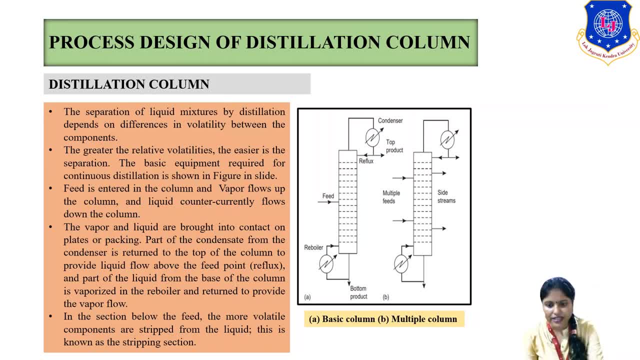 basic column and the multiple column. so what happens in the basic column? that one one feed is there and it gets separated, the we get the top product and we get the bottom product. Top product is known as distillate. so what happened in the basic column is that 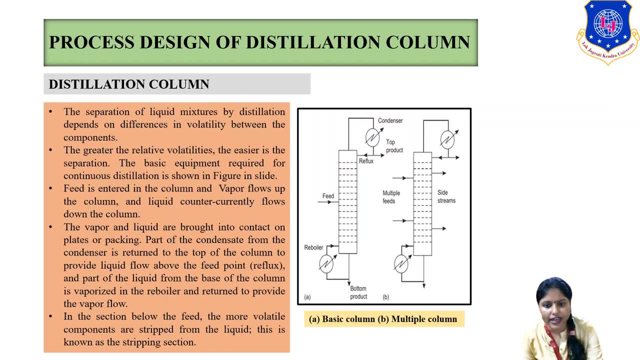 the feed is entered into the column and we get the top product and the bottom product, while most of the top product we don't get from the top product. we just take half of the top product and we reflect it back means we use some of the top product which has high volatility, which has 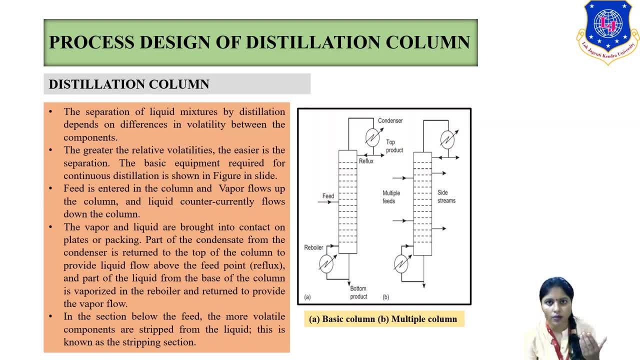 very good product and which has a low boiling point. right, and that will. we will again reflect it back into the column. While in the bottom product, what happens as a re-boiler is kept, some type of heat is generated and due to that, the vapor has been formed and it goes to the 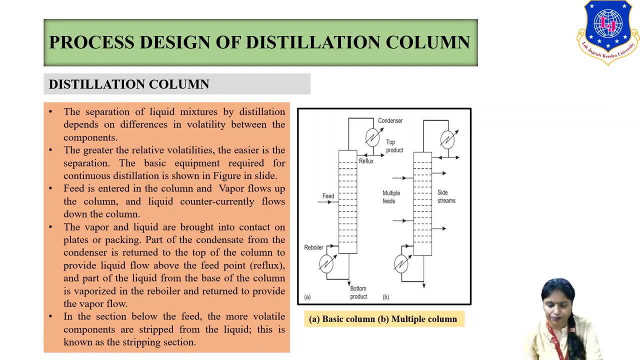 condenser. the rest it goes to the bottom product. and what happened? the multiple column. in the multiple column we can see that there are two types of feed has been fed into the column and we get same, the top product and the bottom product based on the volatility. So let's see to the 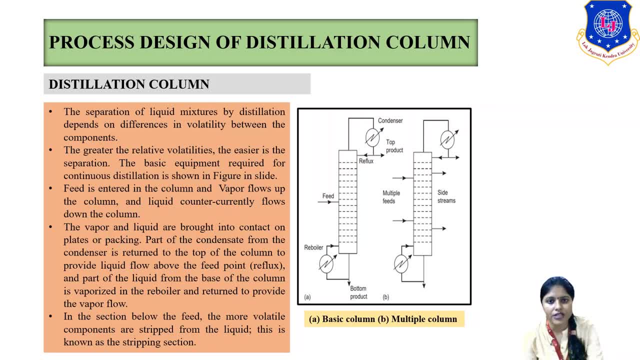 definition of the distillation column that the separation of liquid mixture by distillation depends on the different volatility. right? so due to its volatility, the difference is been done, the separation is been done between the two column and if they they have the greater volatility, then it is easier to get. 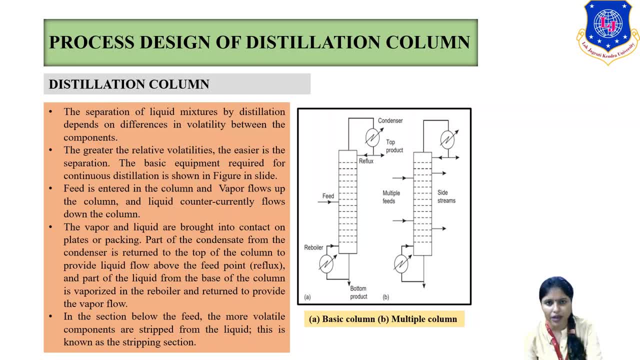 separated. so if now the question arises, ma'am, how, if there is a low, less boiling point between the two liquid, then if this, can separation be done? yes, it can. separation can be done due to the distillation, and it is also known as azeotropic distillation. so we will see to. 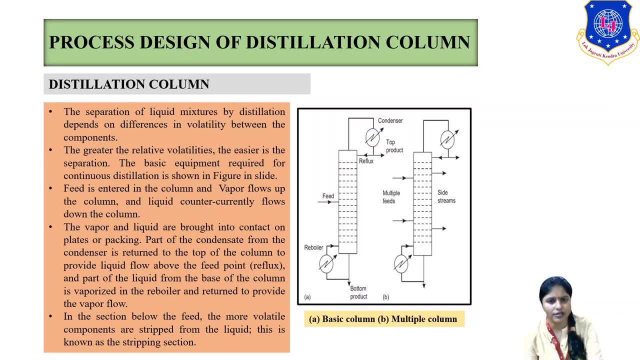 the later part, that what is azeotropic distillation? but the if the boiling, what is very near it to each other we use. the zeotropic distillation means we use one and trainer to it and one of the entrainer will get mixed tool, one of the liquid act. the separation can be done right. so, moving on the 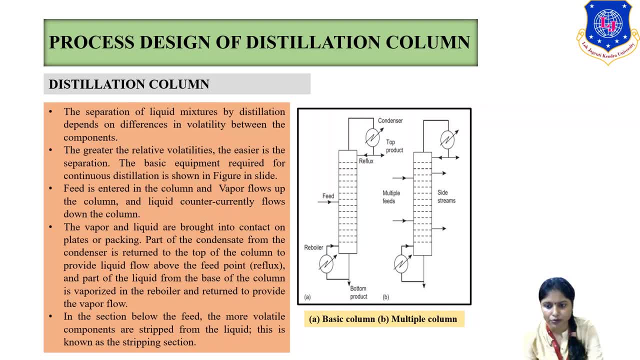 basic column that the furnace entered in little bit volume and the vapor flows out to the column and the liquid counter pulsing flows onto that column. while the vapor and the liquid are liquid are brought into the contact on the place and of the paddling and some of the part will be. 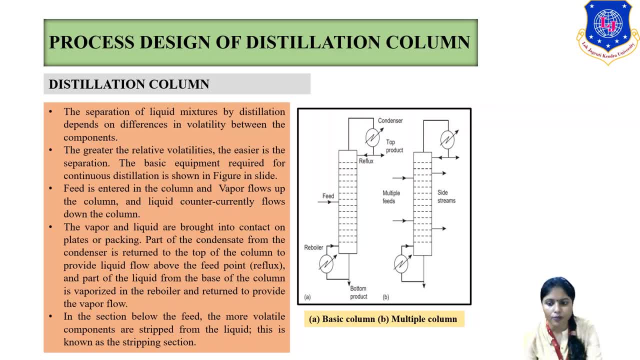 moved to the reflex in the selection. below the feed, the more volatile components are spread from the liquid and this is known as stripping section. so there will be two types of section: above the feed part- it will be known as rectifying section, right and below the feed. 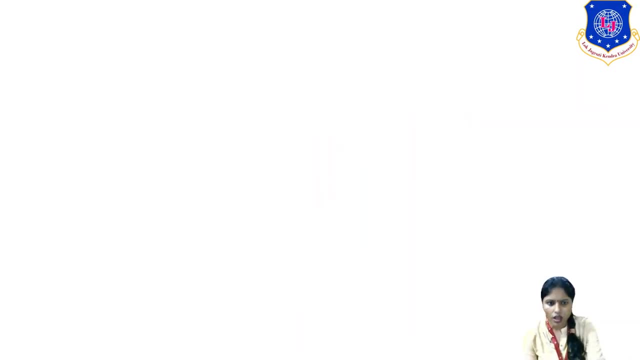 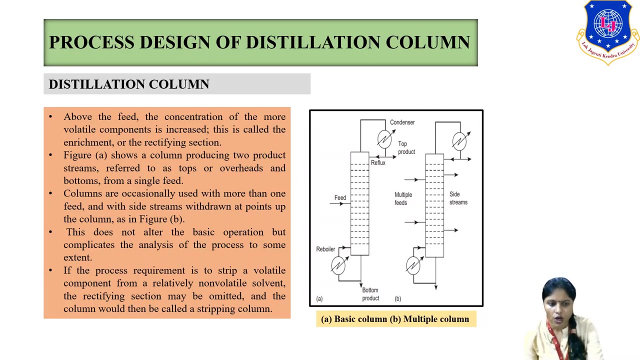 part, it is known as stripping section. moving ahead that in the distillation cursor operations the top product is required as a vapor. only the sufficient liquid is condensed and provide the reflex flow to the column, and the condenser is also known as partial condenser. so what happened? 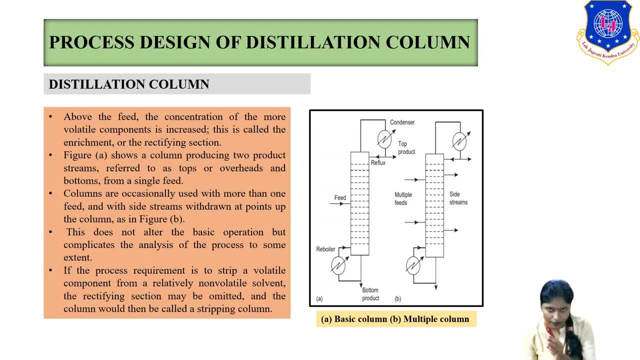 over here that i have already told you that some of the part is been reflected back to the column right. so what happened? that if some of the part is been reflects back, or some of the part has been compared to the column back back, then it is known as partial. 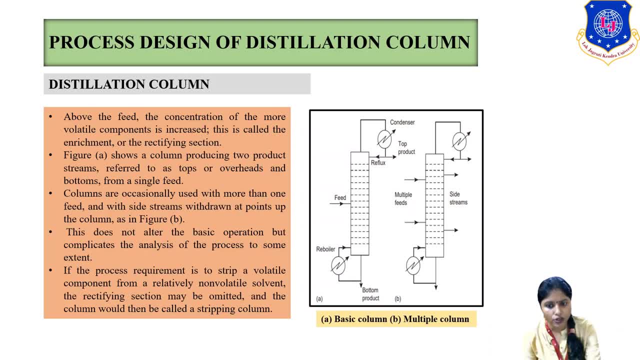 and if we don't want the product and we are feeding it back to the full top product, back to the column, then that is known as total condenser. so first when we start the distillation column or any operator start the distillation column, as the first timer always the total condenser has been used means we don't take the product instantly. 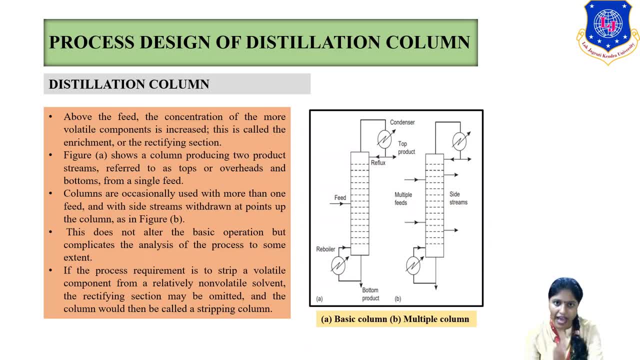 right. so to achieve the targeted product, we have to fed back into the column, so at that time the condenser is being used right. so, above the feed, the concentration is more of the volatile components increased, and this is called the rectifying section, as i have told you, the fed is above the 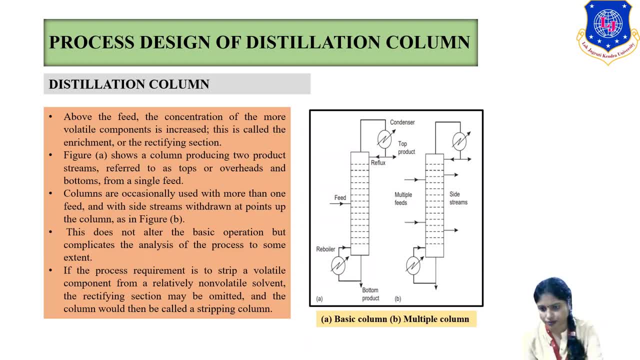 fed, it is a rectifying section and below the fed it's a stripping section. so the figure a shows that the product has two streams, which is referred as overhead, and the bottom bottom which and the basic column. it is a single feed, while the column columns are occasionally used with more than one. 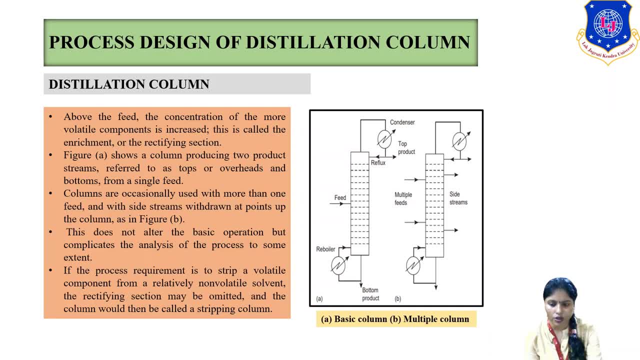 feed and with tight stream we draw a point, a point up to the column, so this will not alter the basic operation, right? so it will complicate the analysis of some of the extent if that in the process the requirement is required to strip the volatile component from a relative non-volatility. 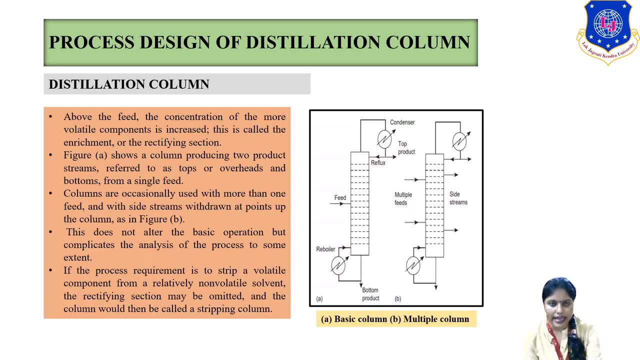 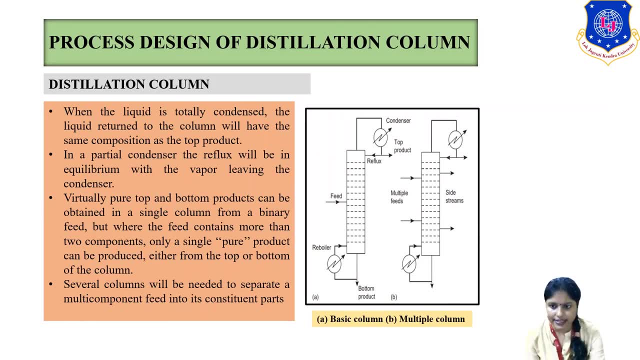 component so and the column can be called as a stripping column. moving on to the distillation column, that that when the liquid is totally condensed, the liquid retention rate is not. Goodbye back to the column, which will have same composition of the top product as I have. 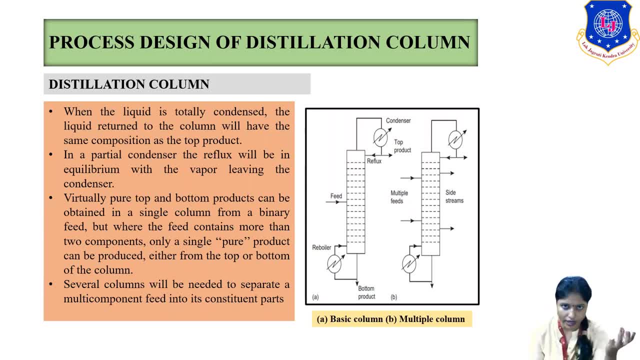 already discussed earlier that if we don't want any top product, so we are at that time. we don't use any top product, we totally get reflex back to the column and in the partial condenser the reflex will be in the equilibrium with the vapor, leaving the condenser. 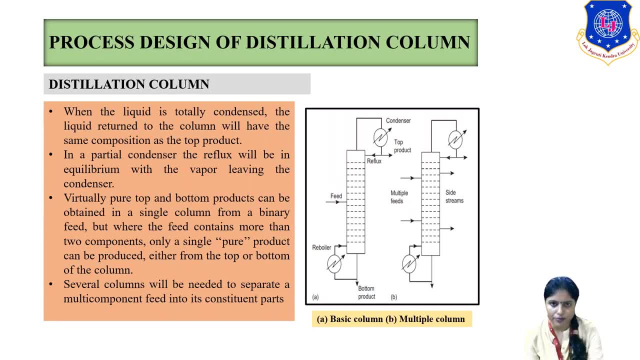 so virtually what top and bottom product can be obtained in single column from a binary field. so when the field contains more than two component, a single pure product can be produced either from top or bottom, as it will depend on the consumer and the solid column will be needed to separate a multicomponent fact. 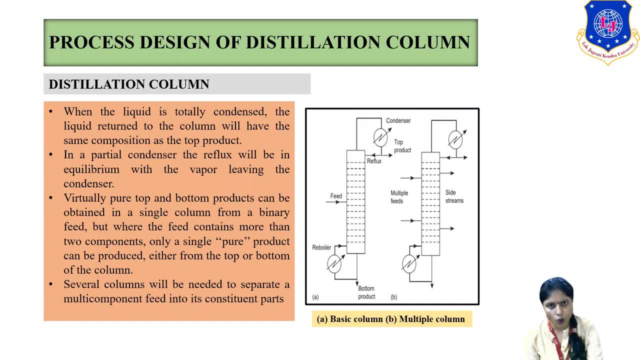 into a constituent parts. so if there are one or more, 2 or more boiling points, rightso, what will happen? that if there are the three products coming simultaneously from the top or bottom, and what happens then? we will again do the separate Rudy process, separation of that product, and then we will take the purity from it. So these are the criteria. 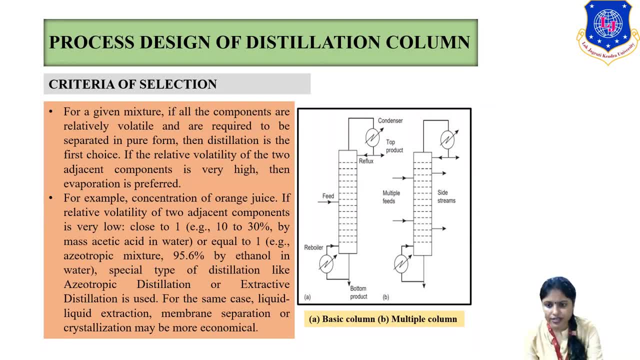 selection of the distillation column that for a given mixture, if all the components are relatively volatile, like and are required to be separated into pure form, then the distillation is the first choice, right? So if we want to achieve a very good product or of higher purity product, then 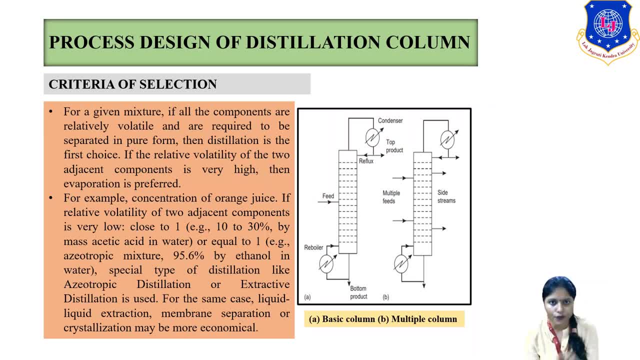 the distillation column is the best equipment used for the separation or for the- we can say that the separation point of two liquids. So if the relative volatility of the two adjacent component is very high, then the evaporation is preferred. For example, the concentration of an 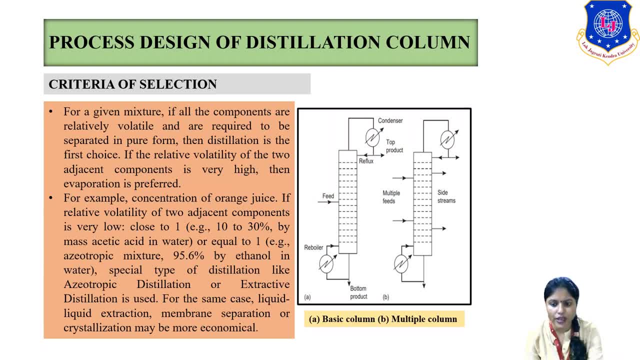 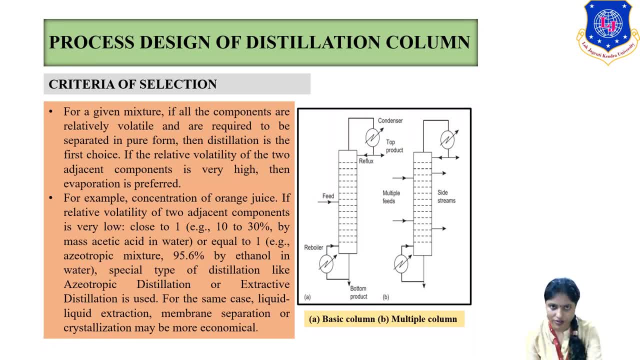 NCO4 or NCO5 or NCO5 or El土 is the entscheiden one product, But azeotropic distillation or extractive distillation is used. I have already told you earlier in one, two, three sentence that what is azeotropic distillation? that when the boiling point is very near to each other. 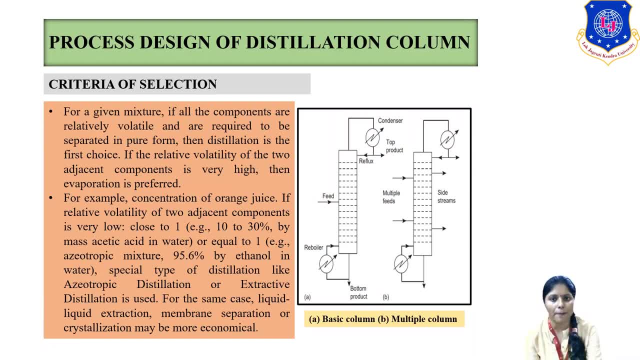 so we don't, we cannot differentiate or we cannot separate that two liquids right At that time point of time. we use the azeotropic distillation. this is also a part of distillation, one type of. at that point of time we use the azeotropic distillation or the extractive distillation. 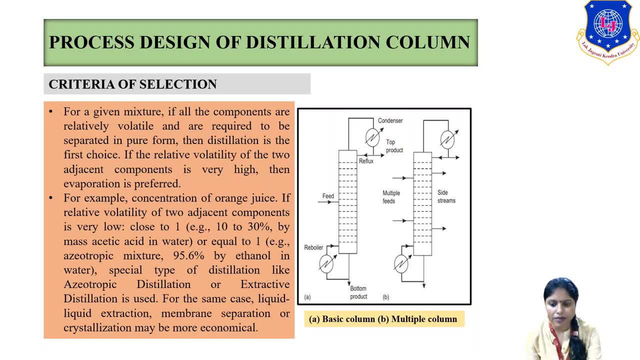 for some case, if the liquid-liquid extraction or the membrane separation or the crystallization may be more economical. so what happened? for example, uh for the separation of pure acetic acid? as you have seen that the pure acetic acid, aqueous acetic acid solution, we use liquid. 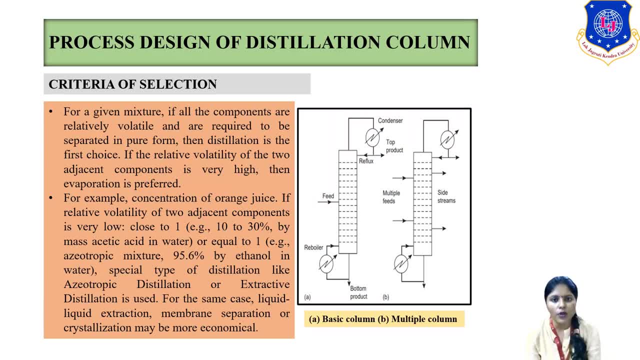 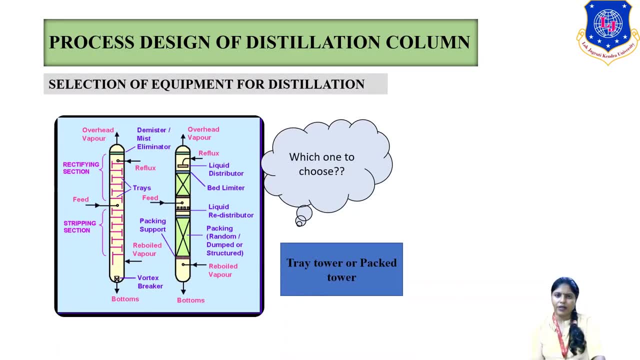 extraction using ether acetate of solvent, which is more economically than the azeotropic distillation. right, and so we will move to the selection of equipment distillation. so what happened in the equipment distillation is that, uh, if the distillation column has been designed right. 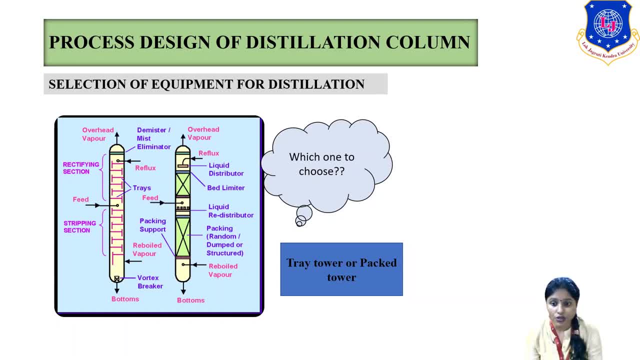 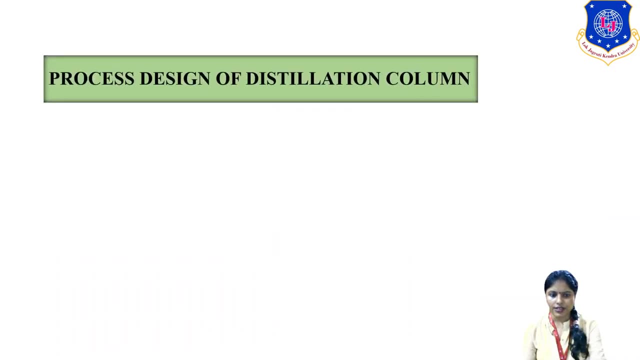 so the first and the foremost question arises is that which type we have to use, either tray tower or the peck tower. so this is a very important uh part, that which type of tower we are using for the distillation. so the next is that, the selection. 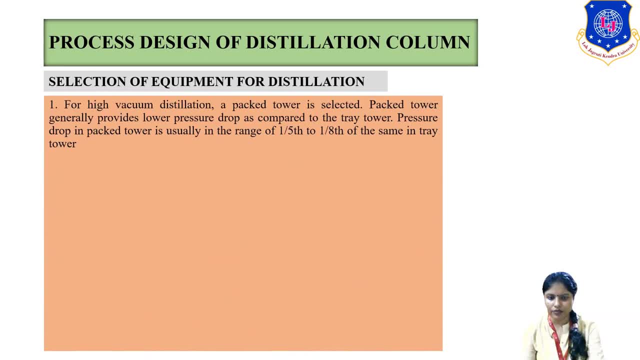 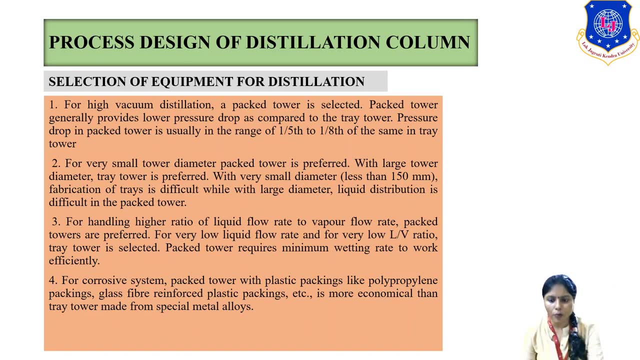 of equipment of distillation is that we can give an example that for the high vacuum distillation a packed tower is selected and the pack tower generally provides a low pressure drop as compared to the tray tower. pressure drop in pack tower is usually as the range of one to fifth to one. 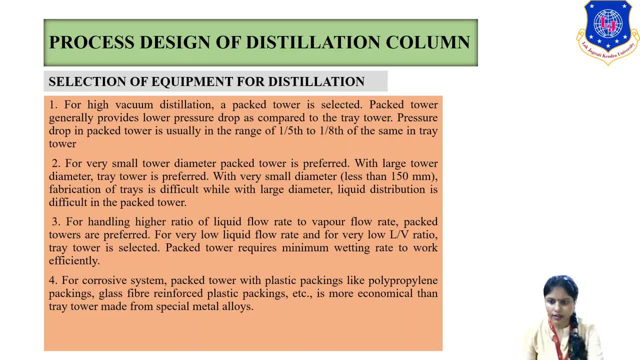 eighth part, of same as a tray tower. while the for the smaller travel diameter, the pack tower is preferred, when the large diameter the tray tower is preferred. so this selection of equipment will you that which type of tower, like tray or pack, to be used and when? so you can see that when the 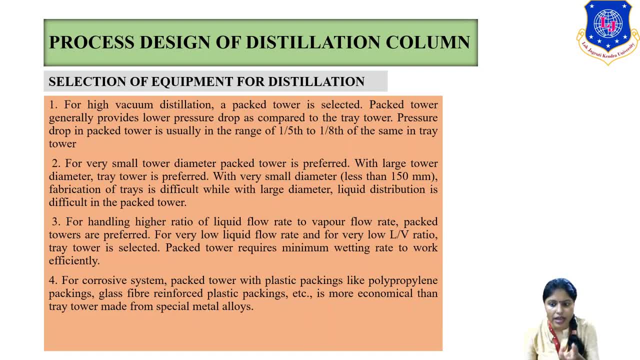 small tower, pack tower is preferred. so with the very small diameter is very less and the fabrication of trace is very difficult, then we usually go for the pack tower because the distribution of the stream will be very difficult. right for the thought is, if we want to handle the higher ratio of liquid, 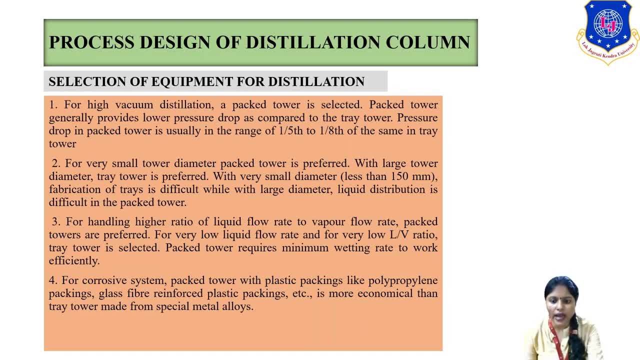 flow rate to the vapor flow rate, then the pack tower is preferred, while in the liquid flow rate a lower to liquid to vapor ratio, the tray tower is selected. so pack tower requires a minimum wetting rate to work efficiently. and the fifth is if the side products are to drawn to the distillation. 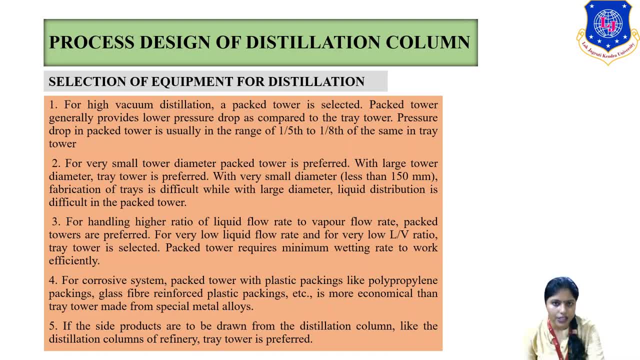 column, like the distillation column of refinery tray tower is preferred. so what happened? the tray tower- you have seen the figure that the tray, the trays, have been kept in between the column right and the between the trays. if we have the different boiling point of each product, 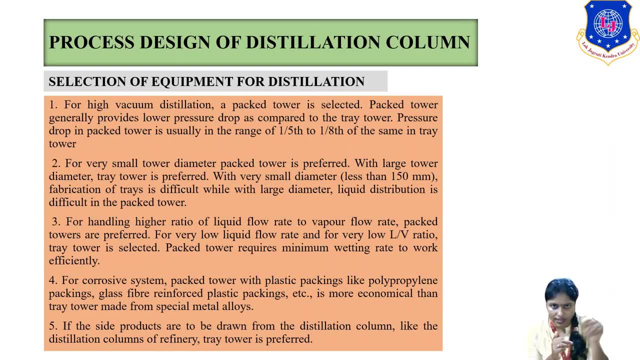 or the each liquid right. we can give a pass bypass from that each of the trays and we can take the desired amount. you have also seen the fractional distillation. distillation, that is the. it is already used in the petroleum industries that most of the crude oils or any different 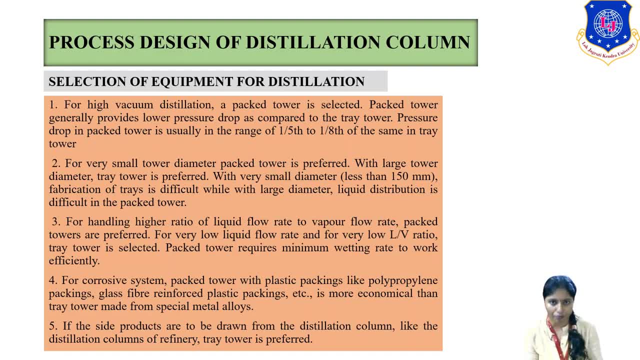 petrol or kerosene on the based on their boiling point has been separated. that had been drawn from the distillation column so in the distillations will be preferable. we can take the direct direct uh desired on type of product from each of the trays and we can bypass it so we can take the. 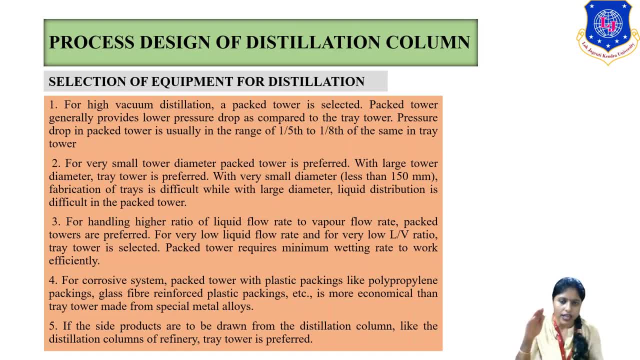 desired amount, while the packing we cannot do, because what happened the packing? it's already packed or in, it's already been enclosed in the column, so we cannot take in between that packing right, the packing distribution will be having a problem to it. we will have. we will have a problem. 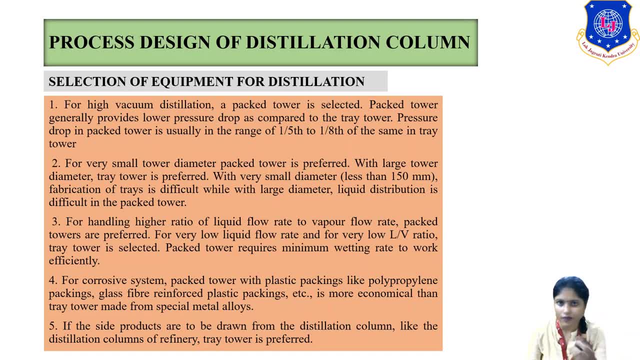 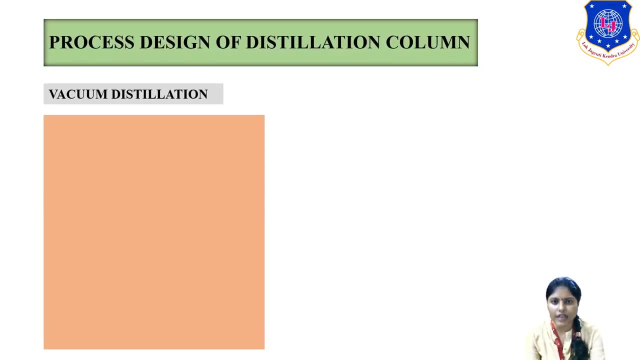 and taking a bypass from the packing. we only get packing products or the packing column. we get the product from the bottom right. so we it's a very difficult for the packing back column. so moving ahead with the one of the type of the distillation that is, vacuum. 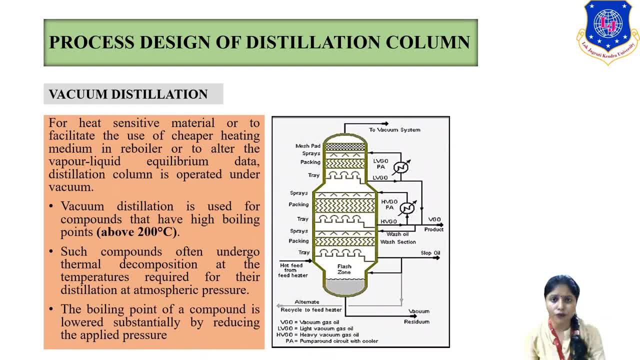 distillation. so what happened? the vacuum distillation that for the heat sensitive material, if the material is very heat sensitive or it's been very uh, heat sensitive means if any point of heat has been given to that material it will decompose or degrade very easily. right at that time we give vacuum distillation. what happens in the vacuum? 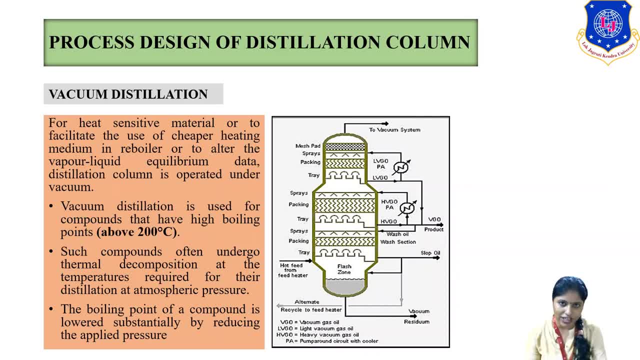 distillation is that when you provide the vacuum distillation, or we provide the vacuum in the distillation, the boiling point reduces. so suppose above water boiling point is 100, right, we, we generally know this right. and if we give a vacuum to the distillation, what will happen? that the 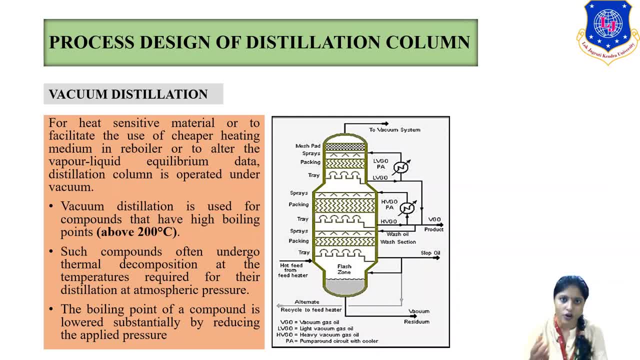 water which is going to the boiling point of 100 or it will get boiled for the first bubble point we can see in the 100 degree celsius. it will decrease to either 60 or 70 as we get give the vacuum to that distillation. so this is a very important part that what will happen? that if we 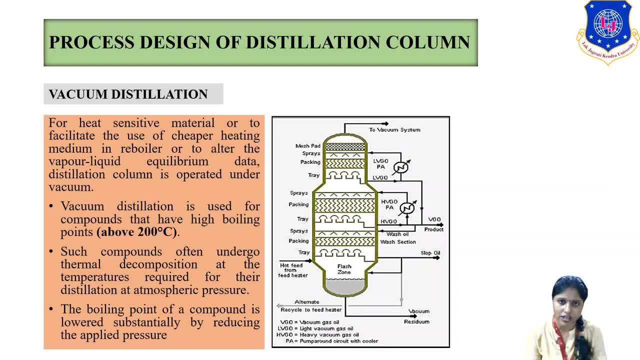 give a vacuum to the distillation, or the vacuum distillation has been used, then the energy or the electricity or the energy consumption will be very less because, as the vacuum is given, the we don't have, uh, the product or the substance or the material doesn't have to reach at their more boiling point. right, they don't have to reach at. 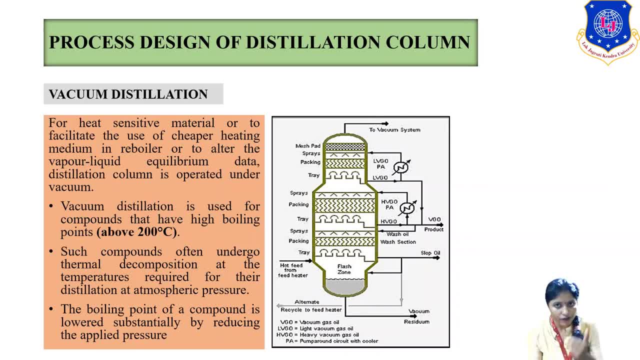 the main boiling point. they have to uh, the boiling point will reduce and they will come again to the lower part of it. right, i have given you the example of water. so if the water boiling point is 100, if we give the vacuum distillation of vacuum distillation, the water has been used. then the 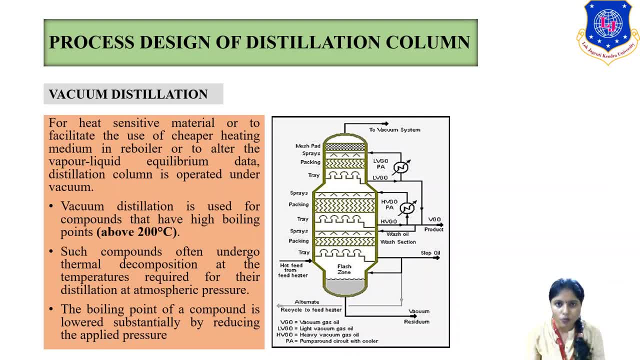 boiling will point will come to 70 to 80. so, moreover, it is a very advantageous to the industry that the economically it will be very viable for the industry and it will be very profitable for the to the industry right. so we will see to it that then the vacuum distillation is already used for. 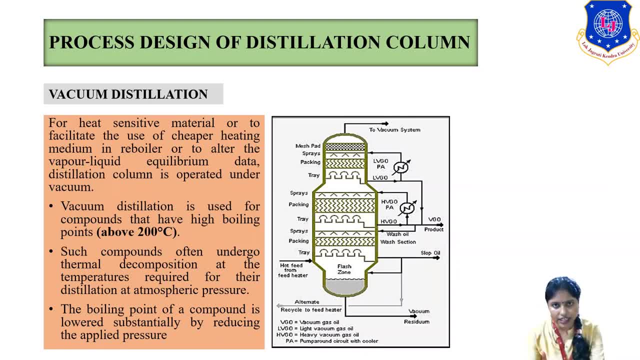 the heat sensitive material, that if its material is very, very sensitive to the heat, then the product degradation will uh form a problem, right, if the degree the product degradation will cause so the product degradation will cause, so at that time the vacuum distillation is used so to facilitate the 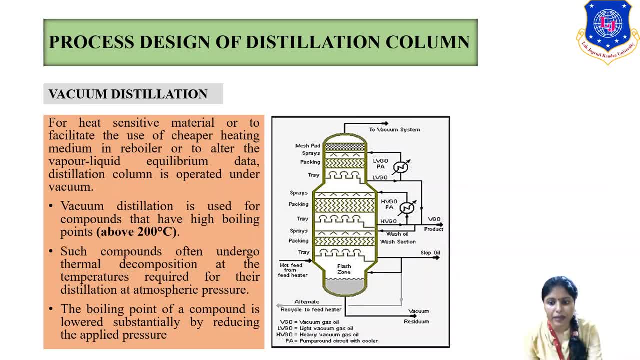 use of the cheaper heating medium in a reboiler to alter the vapor liquid equilibrium rate at the distillation column is operated under vacuum. so vacuum distillation is used for the compounds that has high boiling point, which is 200 degrees celsius, and such compounds often undergo thermal. 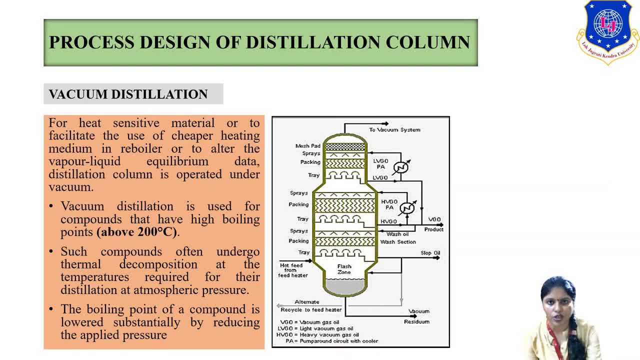 decomposition at the temperature required for the distillation- atmospheric pressure. the boiling point of a compound is lowered subsequently by producing the applied pressure. we can see in the figure. i have given the figure of vacuum distillation right. so the vacuum has been passed, the feed is passed and the vacuum distillation is being Herrmann Hokke here. but though the vehicle temperature seems to be high, it means that theına called till it is higher. so there is no connected 230.6 degrees in this particular option. the water will be drained thereafter, hence it is only used for to warm. 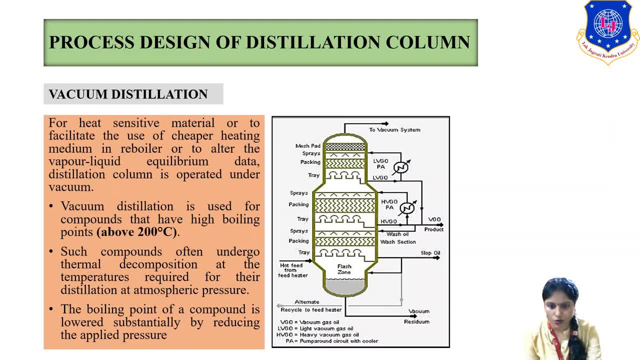 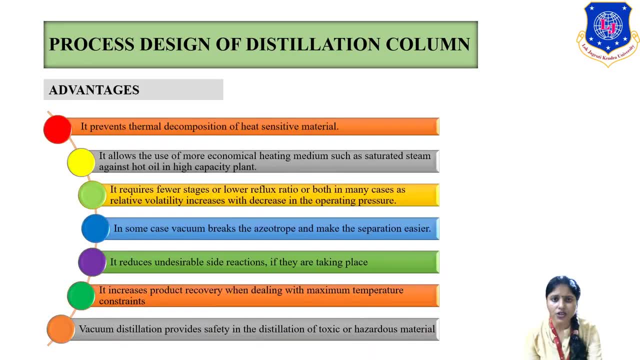 been used. there are many type of trays, packings to be used in the vacuum distillation. any type of packing or the tray can be used that we can the desired compound advantage of the vacuum distillation. so what is the advantage of the vacuum distillation? that the first: it is a thermal. 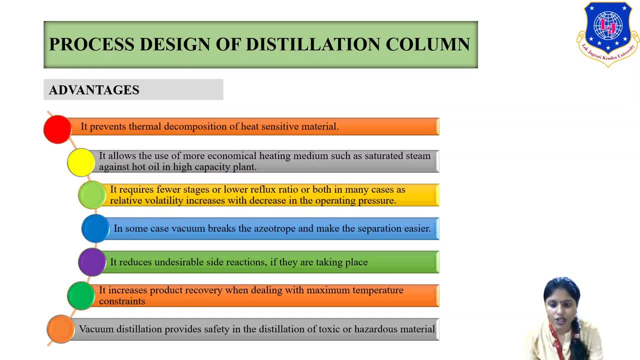 decomposition of heat sensitive material. second, it allows the use of the more economical heating medium, such as saturated steam against hot oil in a high capacity, a plant say. third, it requires fever stage or the lower reflux ratio on both. in many cases that is relatively volatile increases and decrease in the operating pressure. the fourth is it: in the case of vacuum, it breaks the azure. 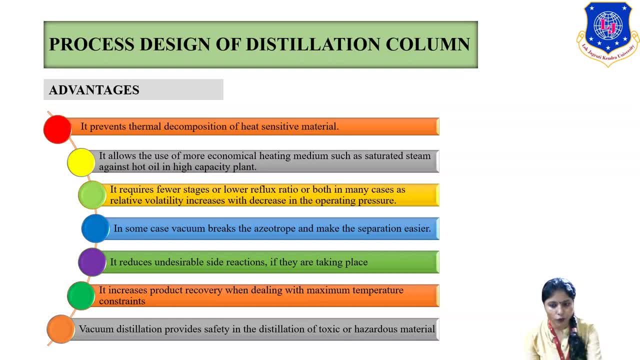 drop and make the separation easier. so the fourth point is very tricky, isn't it that in the azure drop, i have already told you, if the boiling point is very nearer to each other, we use one type of entrainer. but but, but if we use the azeotropic distillation in the vacuum, okay, at what will? 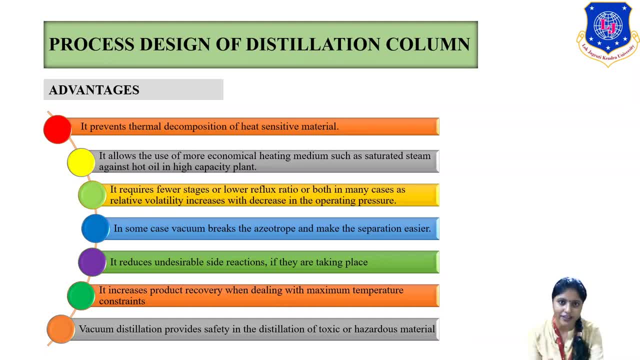 happen, the boiling point which is coming at that part or at that point it's going to boil, it will get produced. so obviously it will get this distillate very easily. so for the breaking of the azeotropic type of liquid or isotropic type of compound we can use the vacuum distillation. it will be very